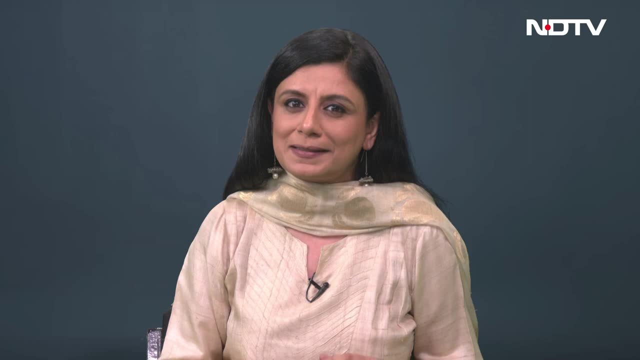 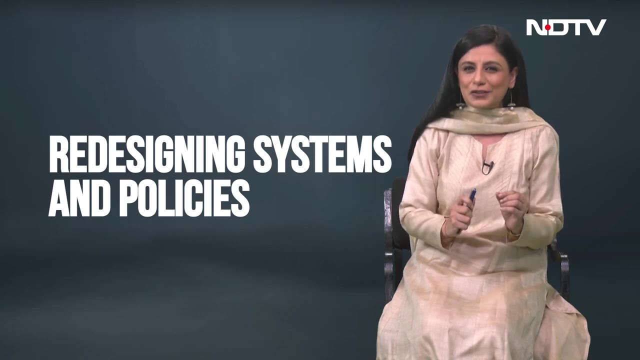 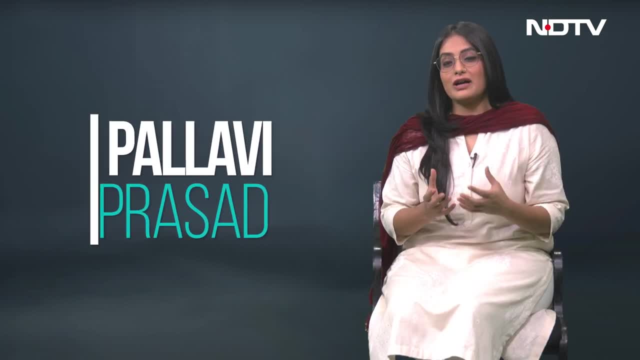 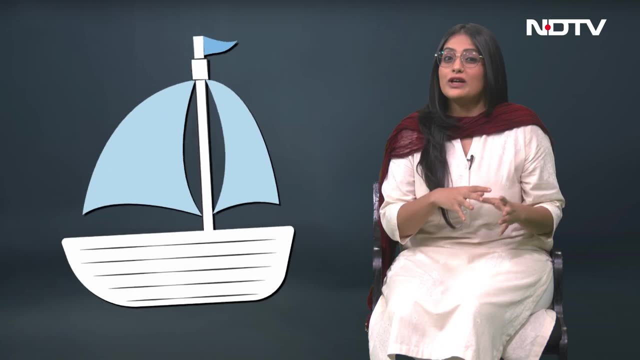 Now, if adaptation is about bailing water from our sinking boat, think of resilience as reinforcing the parts of the boat that haven't yet been breached or weakened because of the water, So that if or when the water gushing in hits those parts, it's going to be able to push the water. out of the boat, And that's why we're here today. We're here today to talk about the protection of water. We're here to talk about the protection of water And we're here to talk about the protection of water. the impact is reduced and we can recover faster. 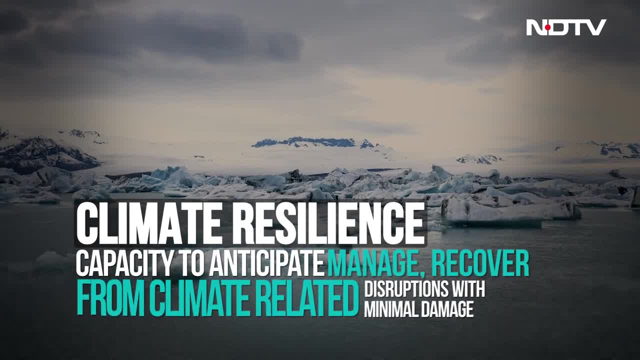 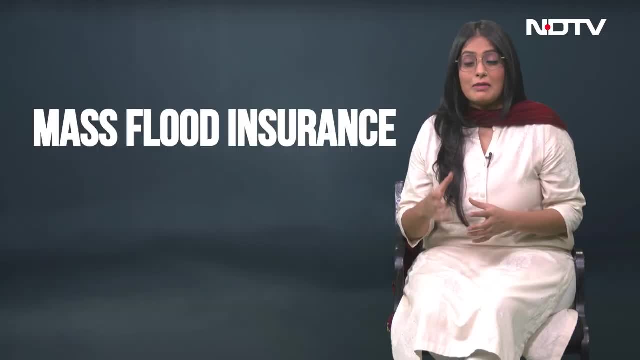 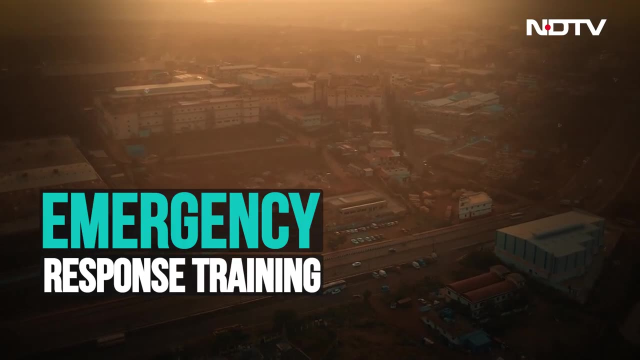 In the context of climate change. this refers to innovations in planning so that communities can bounce back quickly from disruptions when they are hit. Resilience can look like mass flood insurance, Allocating resources to disaster preparedness, such as emergency response training, stockpiling essential supplies and establishing temporary shelters. 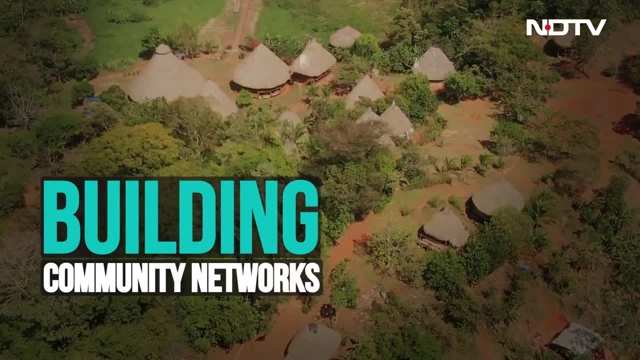 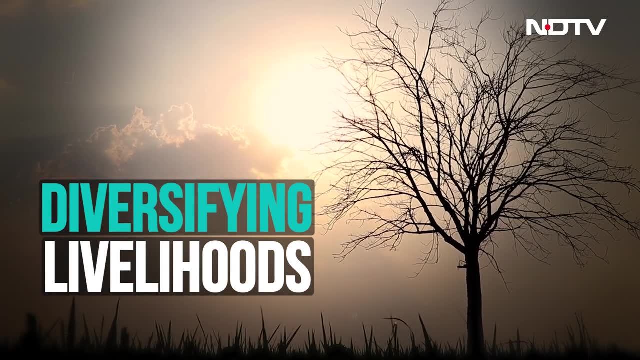 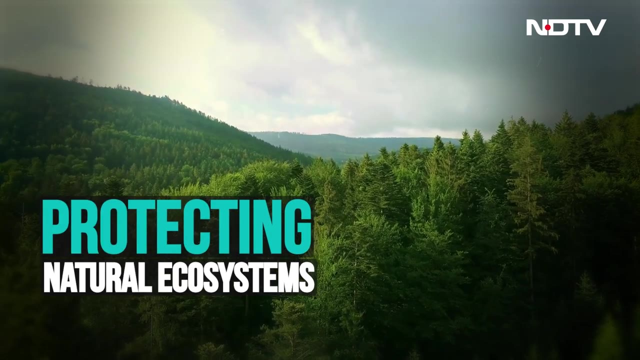 Building strong community networks that can provide assistance during and after climate-related events. Diversifying livelihoods to be less dependent on a single sector or activity that may be hit by climate change, Or protecting and restoring natural ecosystems like forests and wetlands that can provide natural buffers. 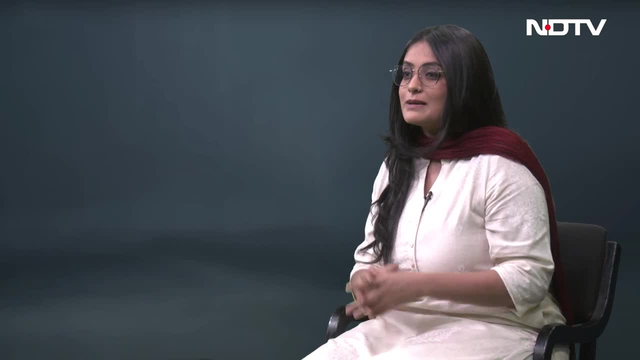 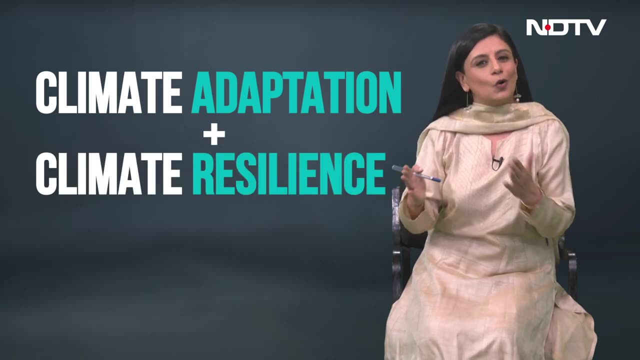 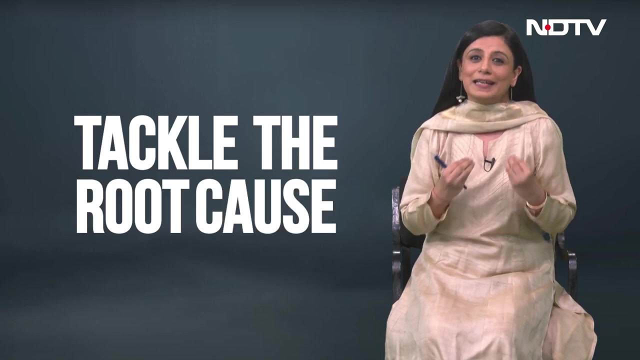 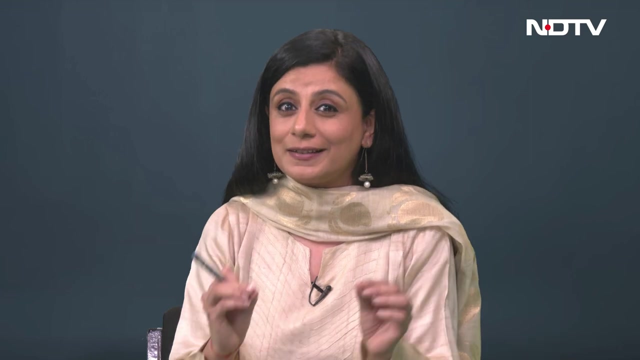 So, in one line, climate resilience means better, more durable, climate-proof systems. Of course, adaptation and resilience need to go hand-in-hand with mitigation to tackle the root cause of climate change, that is, our global heat-trapping emissions. Which is to say that if we want our boat to stop taking on more water sooner rather than later, 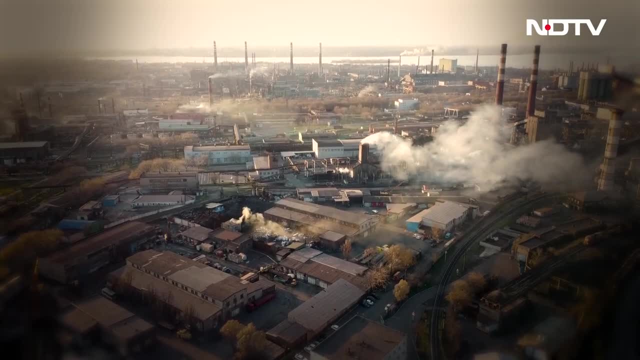 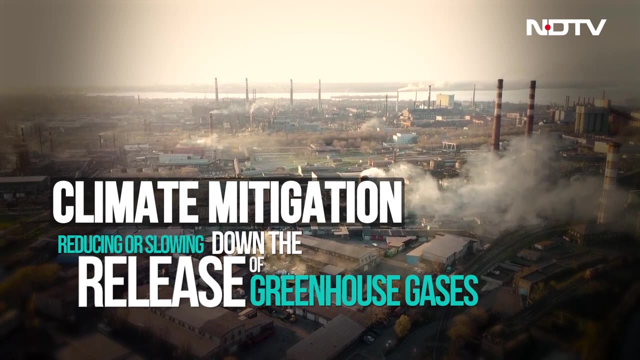 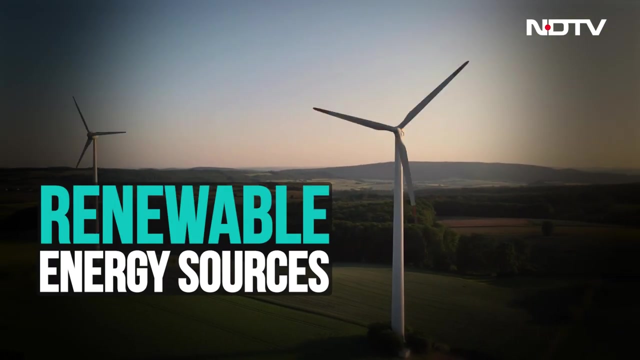 we'll have to patch those leaks Now. in the context of climate change, mitigation means reducing or slowing down the release of greenhouse gases into the atmosphere. We can do this by shutting down coal and gas plants, using renewable energy sources like solar and wind power.